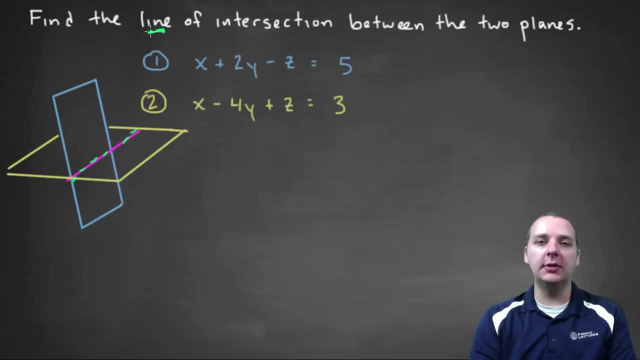 is our answer even going to look like? Well, you remember when we discussed lines in space. these guys are usually written either in symmetric form or parametric form. I kind of prefer parametric form. That's where you have the X and the Y and the Z value written in terms of a parameter, usually like T. 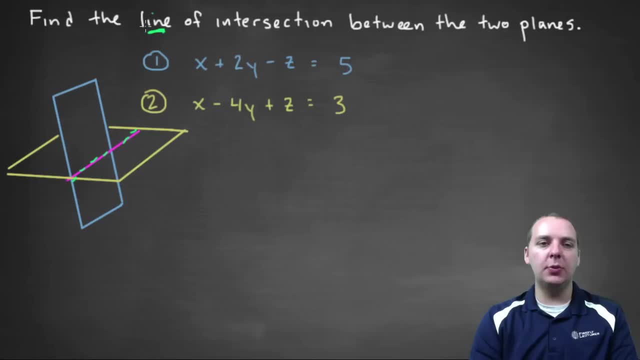 independent of the line of intersection between these two planes. So we're going to be trying to find two very similar lines, independently of one of one another. So that that's what we're going to try to do. So we're going to try to find a set. 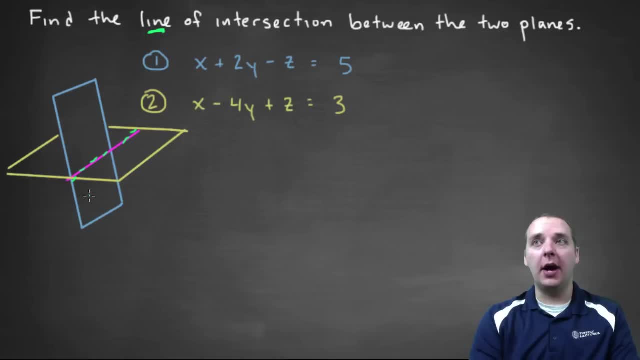 of three equations: X and Y and Z, in terms of a parameter T that represents this pink line right here, Right now. how are we going to make that happen? How? how does that work exactly? Well, we're going to treat this guy almost kind of like a. 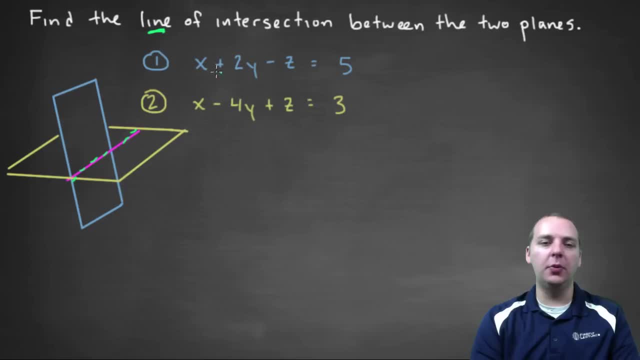 system of equations, because you've got two equations with three unknowns and Z or somebody easy to solve for, and both of these guys, and set them equal to each other and then kind of go go from there So that if we can get X, let's say as a function of, let's say like Y um Z as a function. 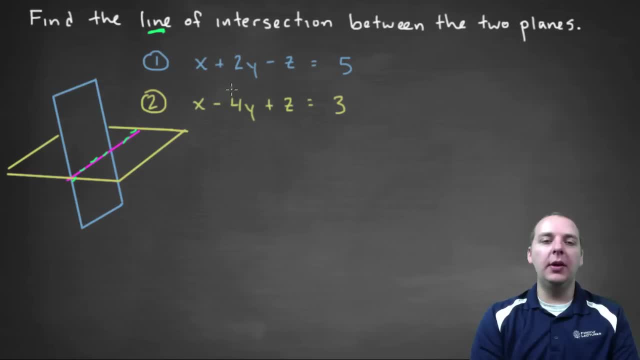 of Y and of course Y equals Y. then we can take the X and the Y and the Z equations and change one of those Y values, let's say, into a T in terms of a parameter, and so then they're all in terms of the same same parameters. 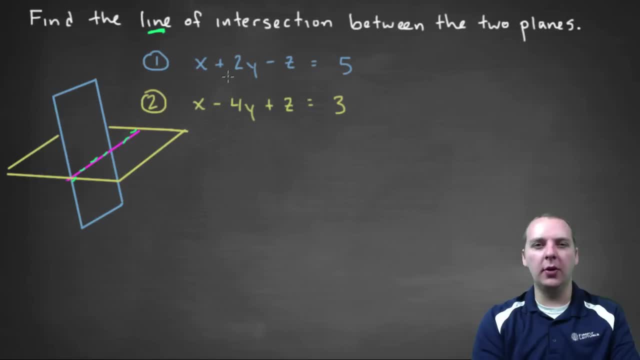 So if that's unclear, don't worry about it, you'll see where we're going as we kind of work through an example. Alright, so let's, let's start maybe by solving both of these guys, for, let's say, X. 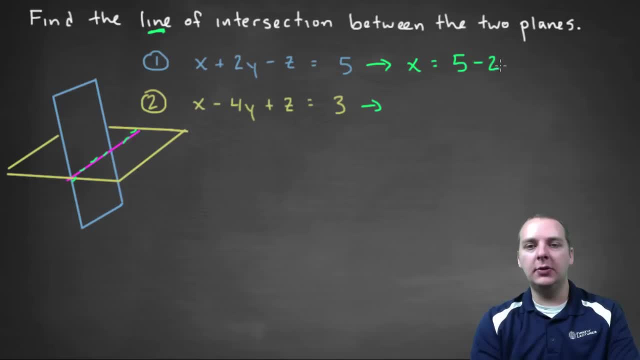 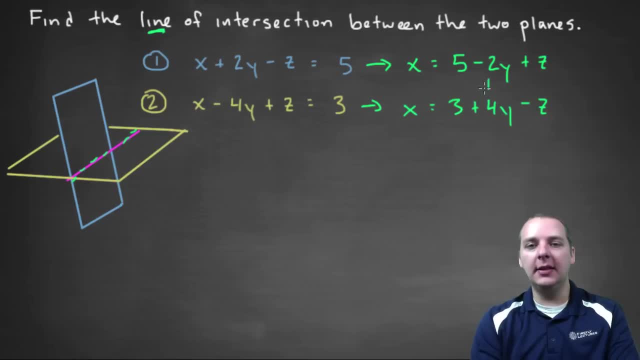 the, the, the. this is X and this is X. that means that these two guys must be the same. If they're both X, then these guys must be equal to each other. So let's take these two right hand sides, set them equal to each other. 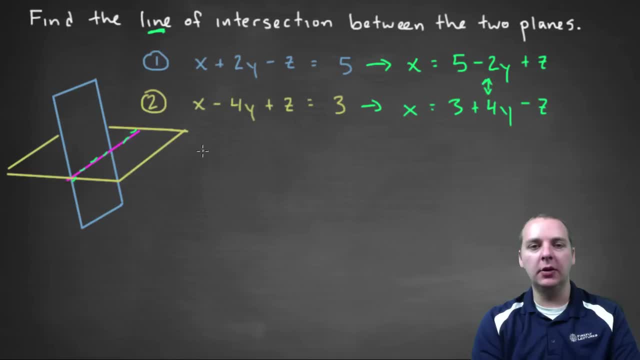 Now I kind of change colors as we go so we don't don't get confused. We'll have five minus two Y plus Z, equal to three plus four Y minus Z. And let's, let's try it again. let�s try to maybe shuffle some terms around. let�s maybe try to solve for Z. so if we 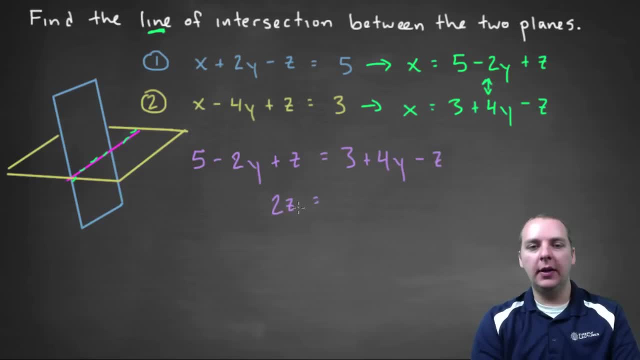 add Z to the left, we get 2Z. if we add 2Y to the right, we get 6Y, 4Y and 2Y makes 6Y, and then 3 minus 5 is negative 2, so it�s looking good and therefore Z would be equal. 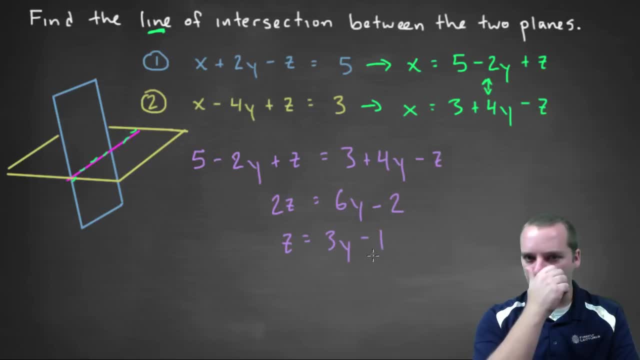 to 3Y minus 1, if we divide everything through by 2, of course. so let me box this in here real quick. so Z is a function of Y. obviously Y equals Y, and now all I have to do is get. 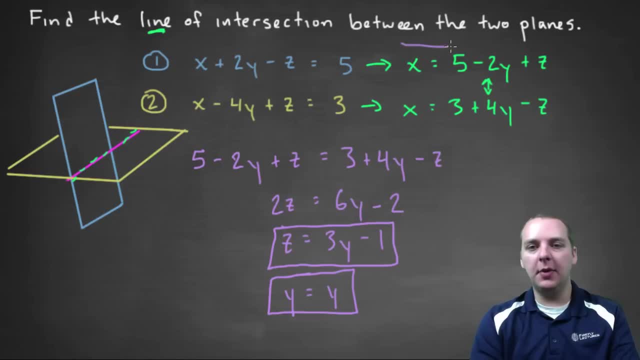 X as a function of Y. but now think about it. let�s just take maybe like this equation right here: X is equal to 5 minus 2Y plus Z, but Z is a function of Y, so Z is equal to 5 minus 2Y plus Z. and now all I have to do is get X as a function of Y. but now think. 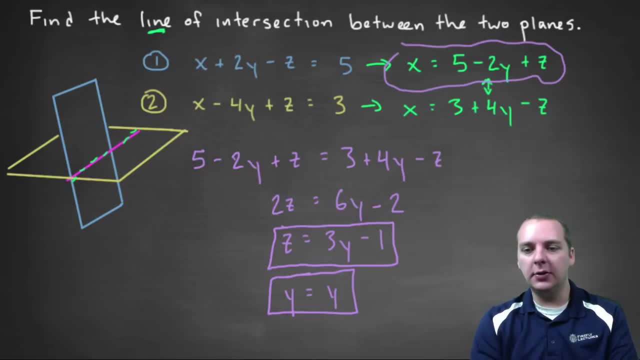 about it. let�s just take, maybe, like this equation right here: X is equal to 5 minus 2Y plus Z is a function of Y. so here, let me change colors here real quick- this Z right here I�m going to replace it with what I know Z is equal to, in our case, 3Y minus 1,. 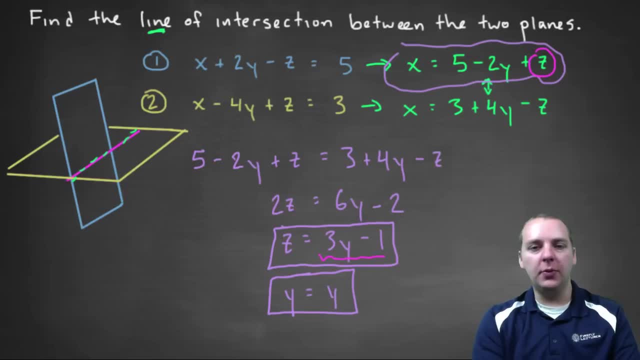 so let�s see here. I�m kind of running out of colors here. I�ll do it in orange. we�ll try to squeeze this in. so X equals 5 minus 2Y plus Z, but we�re not going to write. 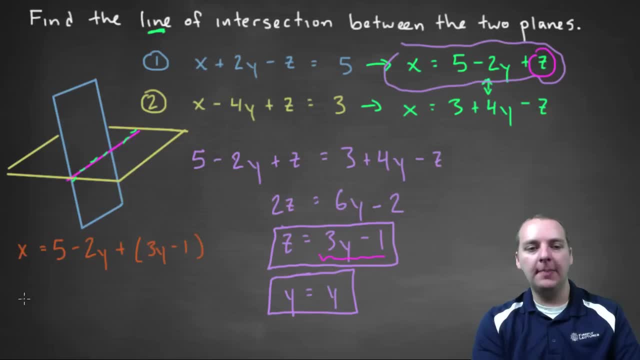 it as Z. we�re going to write it as Y. so X equals 5 minus 2Y plus Z. but we�re not going to write it as Z. we�re going to write it as 3Y minus 1, clean that up a little bit. 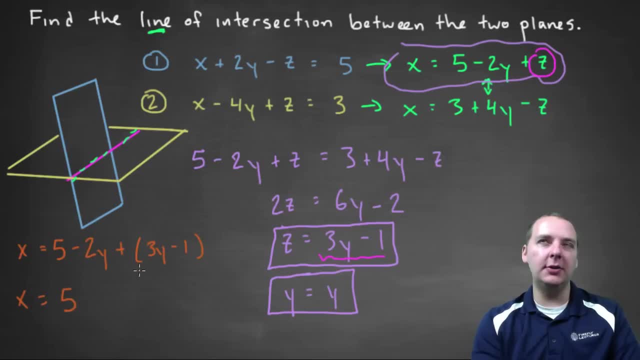 and we�ll get 5,. let�s see: minus 2Y plus 3Y makes plus 1Y minus 1, so X would be equal to 4 plus Y. so there you go. I�ll box that guy in as well. so look at these three boxes. 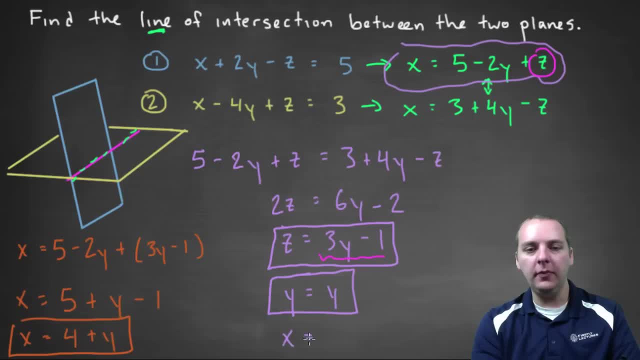 right here. you know, I�ll even write it in purple up under here: X equals Y plus 4, so Z is a function of Y, Y is obviously a function of Y and X is a function of Y. so all we need to do is change these Y's on the right hand side to a parameter T and we�re. 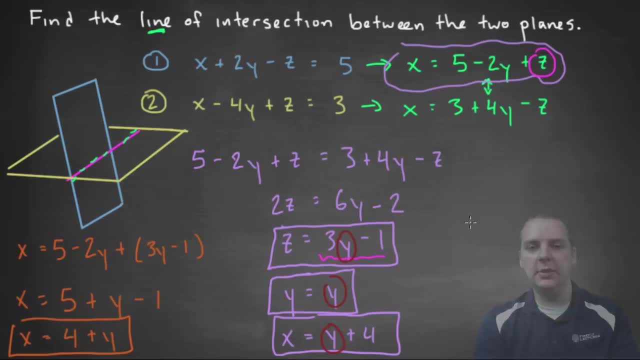 done, so let me squeeze that in right here. I�ll do this in yellow, so we�ll say: X is equal to T plus 4, Y is equal to T, and then we�ll do this in yellow, so we�ll. 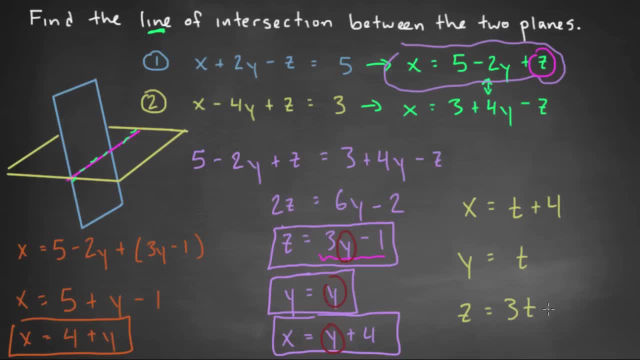 say, Z is equal to 3T minus 1, so basically it works like this: if you pick a T value like 7, let�s say: then Y equals 7,, so Y equals 7, if your T value is 7,, then that�s. 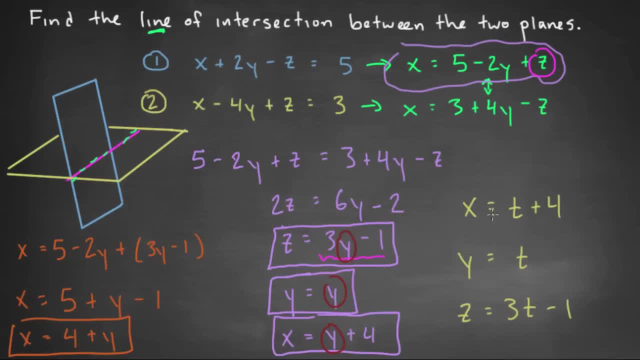 what Y is. but since X and Z used to be functions of Y, but Y is the same thing as T by our own choosing, then naturally X and Z would now be functions of T. right, because T is the same thing as Y. 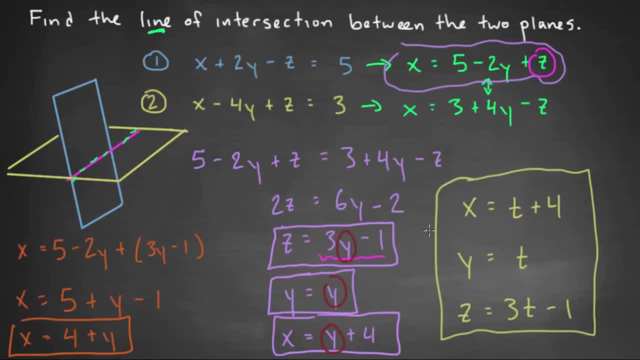 So we�ve written these guys as a set of parametric equations, and this set of equations gives you this line of intersection right here. so these can be a little tricky, it takes a little practice, but basically all you do- just to repeat one more time- is you? 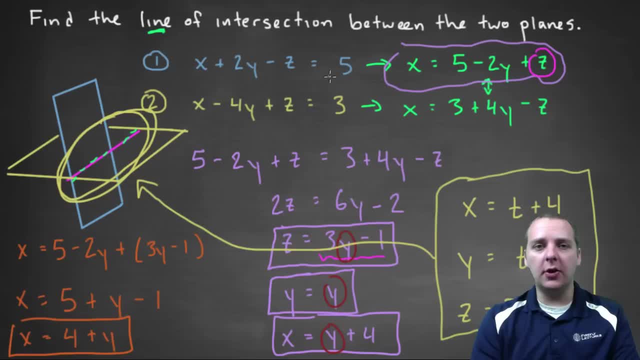 solve for one of the variables and don�t. you don�t always have to solve for X. do whatever is easiest. if you wanted to, maybe you can try this at your desk. maybe solve for Z to begin with And then go that route. that�s fine, but solve for one of the variables, then set those. 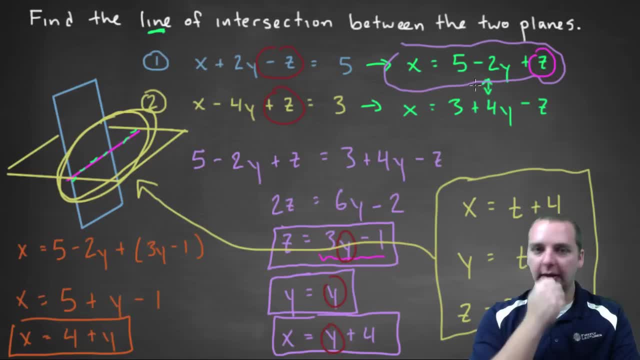 equations equal to each other- the right hand sides- and you�ll reduce the number of variables down and then keep going until the X and the Y and the Z are all in terms of some variable- our example is Y, maybe your example it will be Z, or what have you- and then, once they�re, 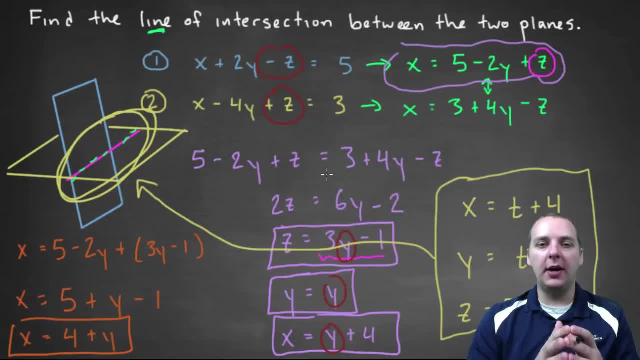 all written in terms of the same variable. change that variable on the right hand side to a T and you�re done. That will be a set of three parametric equations that represents your line in space. If you�d rather it be in symmetric form, I�m not going to do this, but right here,